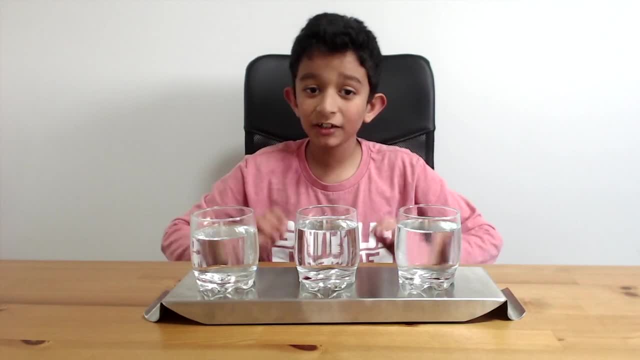 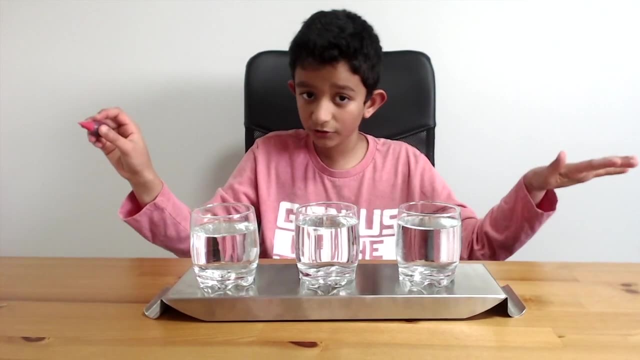 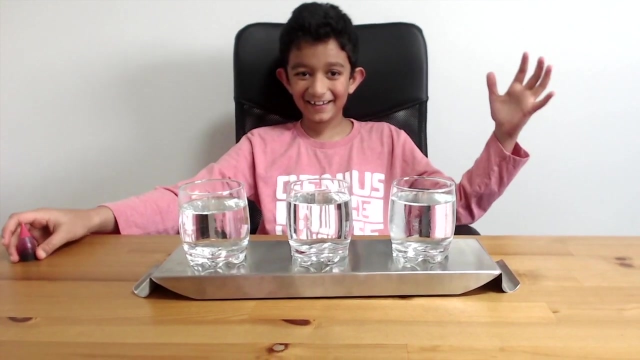 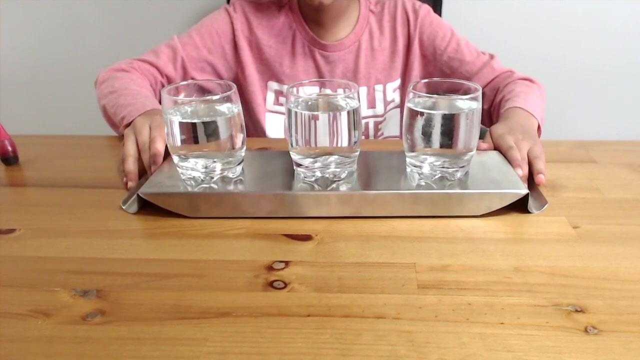 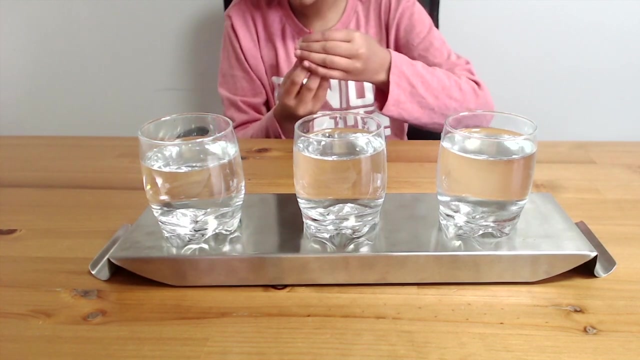 and boiled this one. Now what we're going to do is take food coloring and drop it in, And remember just one drop, Not more than one. One drop of food coloring for each glass. Now let's get started. Now I move this a little closer And it's good. Take food coloring, open it up And one drop. 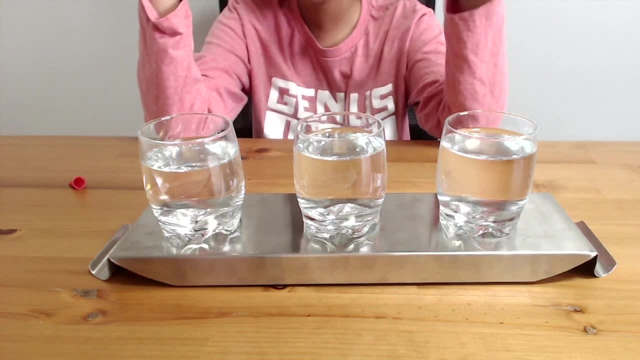 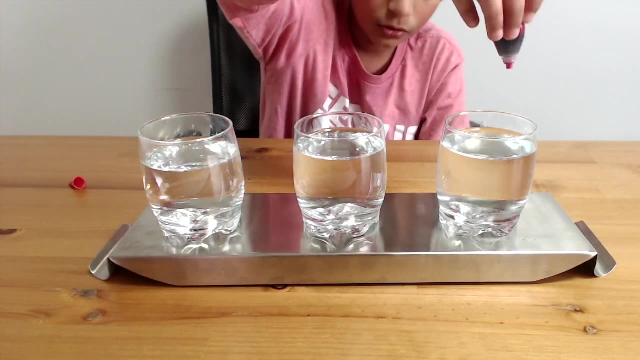 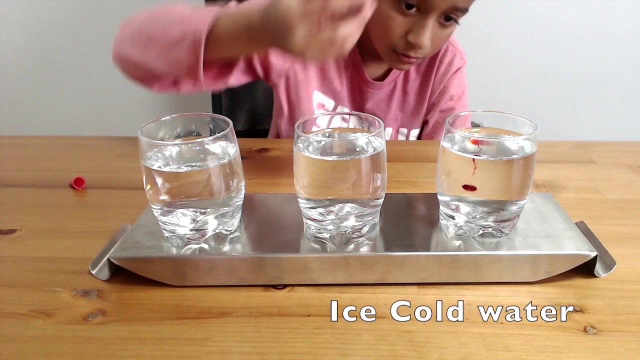 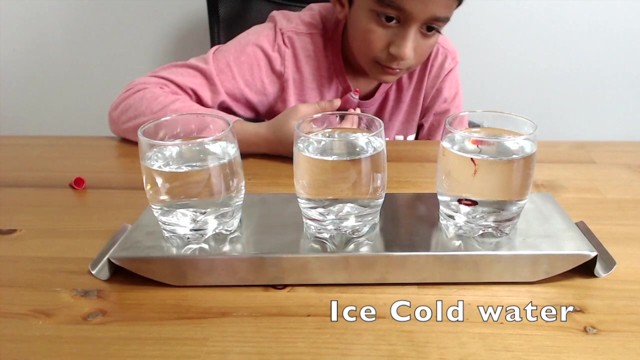 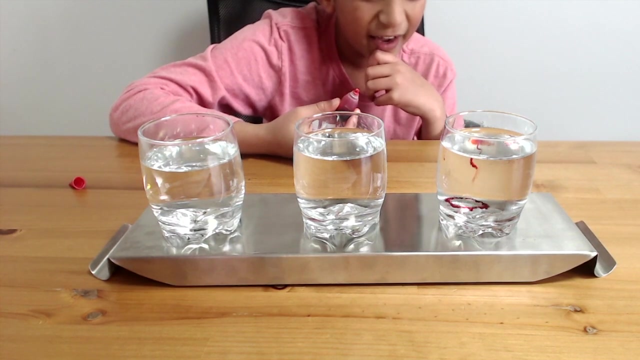 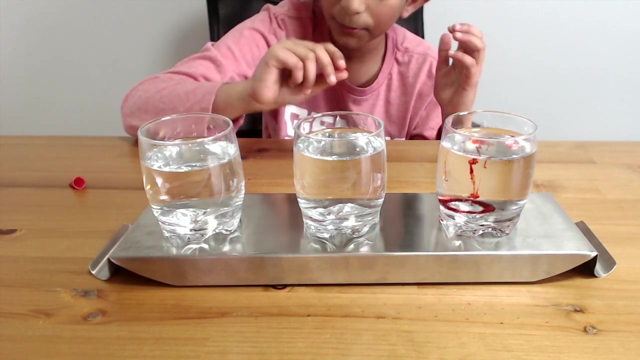 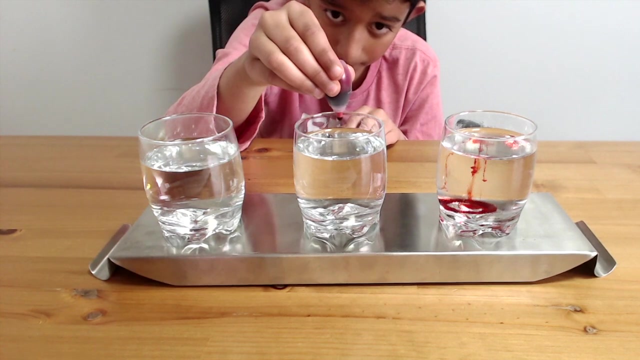 So observe what happens to each of the glasses. Remember Cold, frustrating Prime temperature and boiling hot. Yeah, did you observe that it didn't spread as fast, it just slowly dropped in like a drop. Now, this one room temperature, one drop. 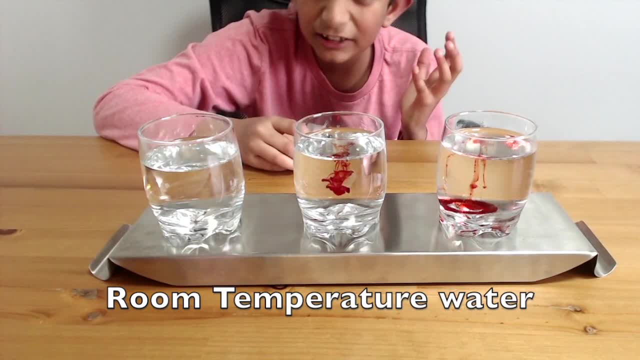 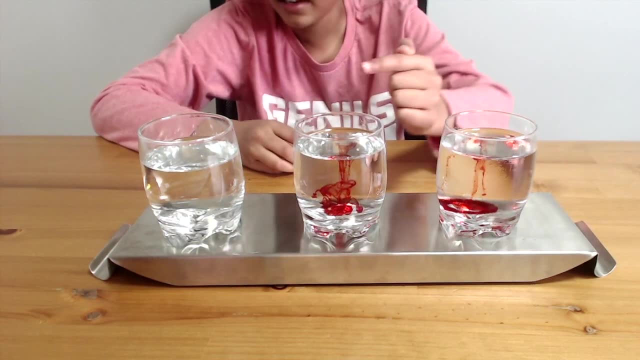 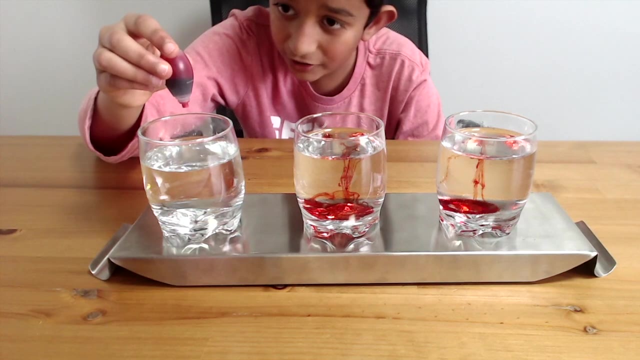 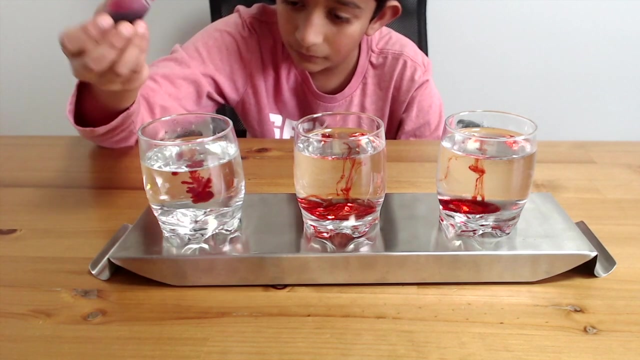 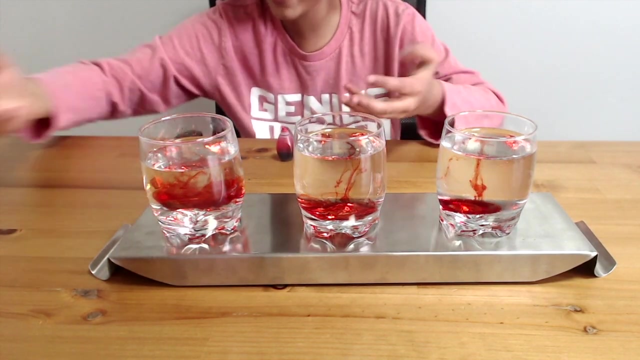 Okay, it spreads a little faster. Look at this. it still didn't spread. Now this one way faster. Now let's try this boiling hot And remember just one drop. Whoa, did you see that? Look, it's already spreading super fast. Whoa, look at this. 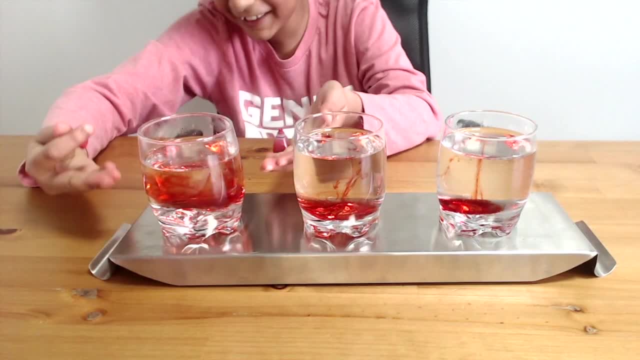 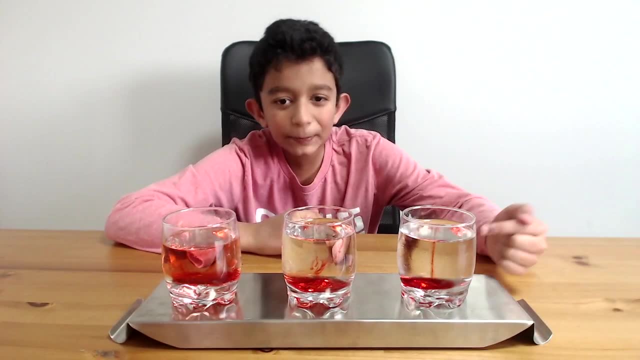 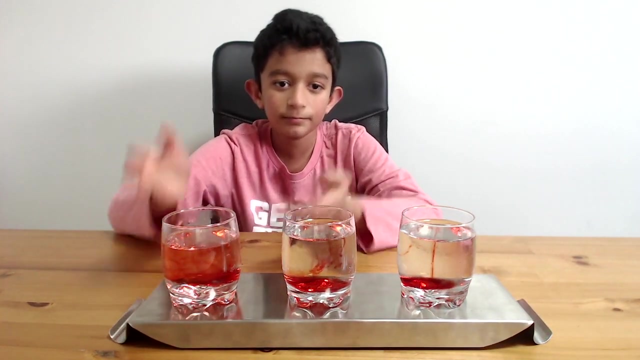 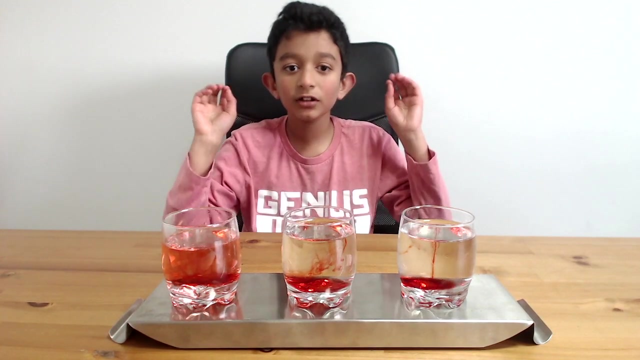 barely Almost. you're already there. Look at that, didn't you? That is just superb. Now keep observing. this is still not spreading. just drop by drop And a little faster And you're done First place. Okay, so this is because of thermal energy, And I'll explain why. So 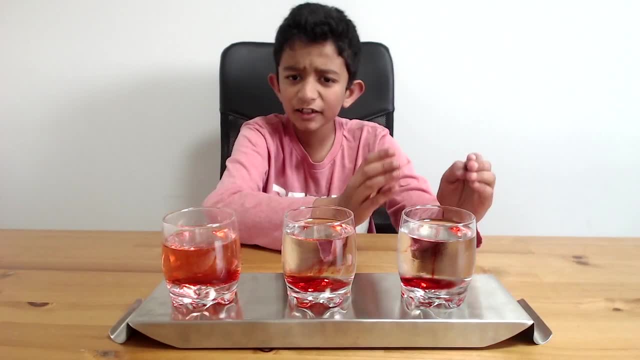 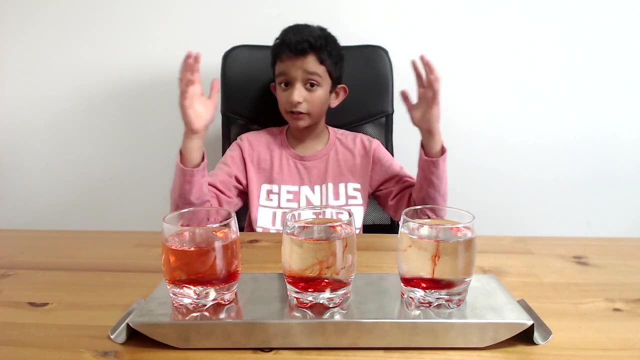 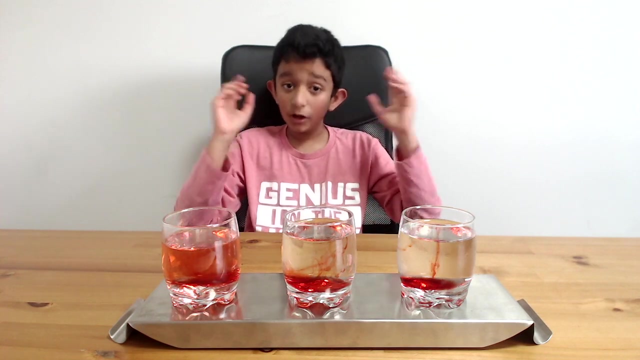 this is cold room temperature and hot. So the water is cold, the thermal energy is very low And remember, when water gets cold it'll start trying to freeze and become solid. So when it's solid, the molecules don't.